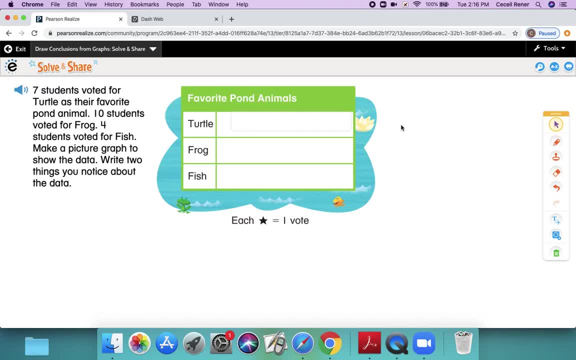 and then write two things I notice about the data. And what data do I have to help us solve the problem? Well, we know how many students voted for the turtle, the frog and the fish, So we know quite a bit already, So we can get started. 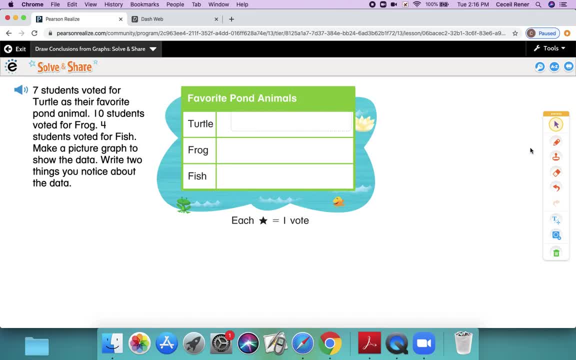 So we have to. let's see what we have to draw here. It tells us that each star equals one vote, So we have to draw a star. So we know that seven students voted for the turtle, So that means I have to draw what Seven stars? 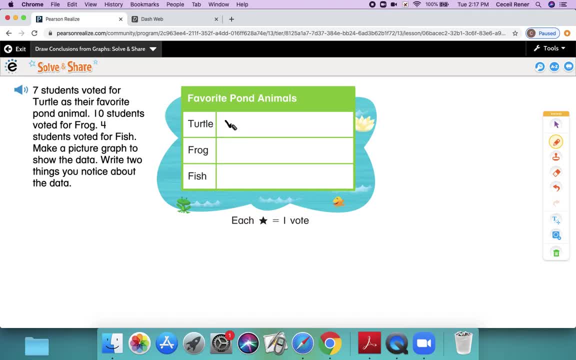 So let's see if I can draw seven stars. So there's one star. They don't have to be fancy stars. boys and girls. That's four, three. Oh, they're getting less fancy as the seconds go on here. They're looking kind of butterfly-like. One, two, three, four, five. 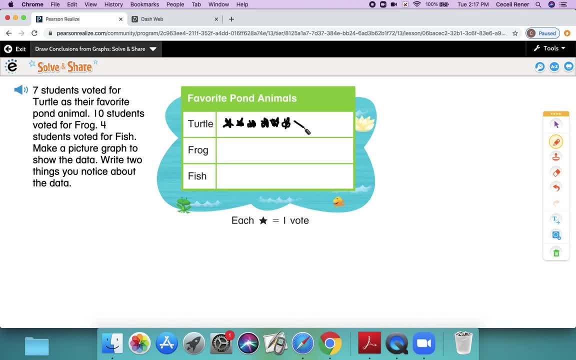 Six, Five, six- I'm going to kind of do the ones like I do on your papers sometimes- Seven, Six Ten students voted for frog One, two, So you guys are drawing these. two. Eight, Four, five, four, three, four, five, six, seven. 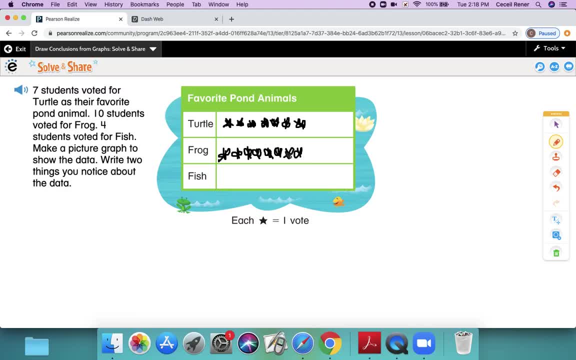 Seven Third, Jaqueline Lおい. Ten, Ten, Twelve, Three, Eight, Nine Grading end anders, 9. Do I have 9?? 1,, 2,, 3,, 4,, 5,, 6,, 7, 8.. Oh, overly optimistic there. 9. 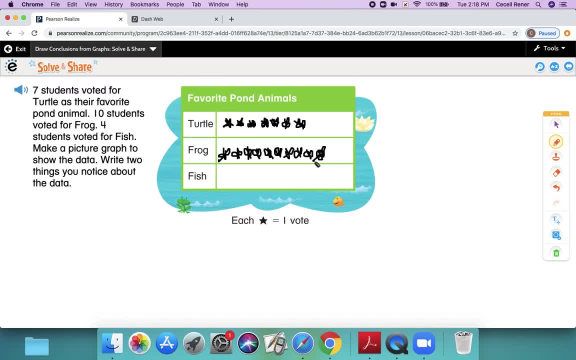 10. And then 4 voted for fish, 10.. Okay, so those are all my very bad looking stars, So let's look Right. two things we notice about the data. So I think probably the first thing that I notice is what 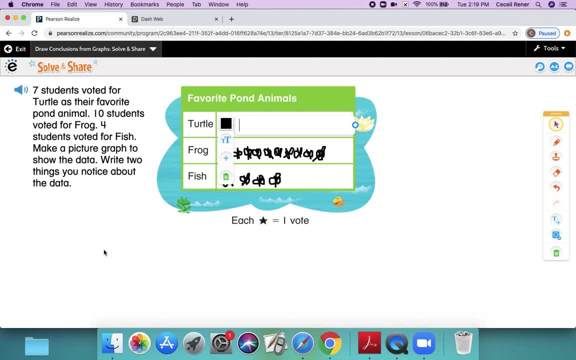 This is that frog has. My first thing I notice is that frog Dog has 10 votes, which is the most of all the animals. So that's one thing. That's the first thing that I noticed is that he has the most of all the animals. 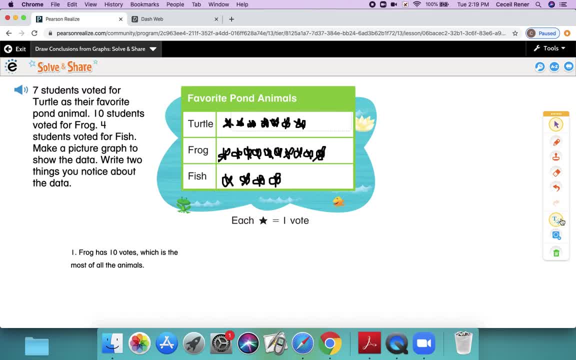 Now, the other thing that I noticed- and you probably noticed this as well- is that Fish is the least favorite animal. And how many votes did that poor Fish get? He only got four votes. Because it votes Because it only has four votes. 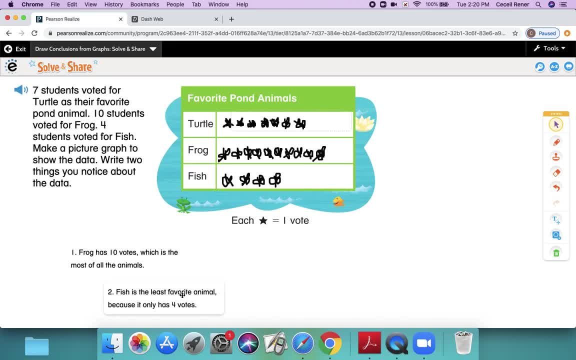 Okay, so those are the two things that I noticed right off the bat. Okay, if you notice something different, you can certainly write down something different, But those are the two main things that I noticed. I noticed that Frog has 10 votes, which is the most of all the animals. 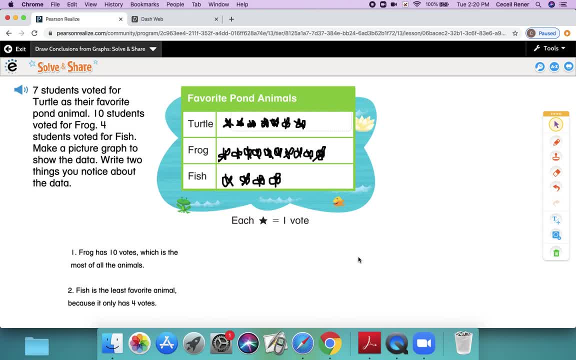 And that Fish is the least favorite animal because it only has four votes. Okay, so now we made a picture graph to show data and wrote two things we noticed about the data. Later in this lesson we're going to draw some conclusions about data shown in picture graphs and bar graphs. 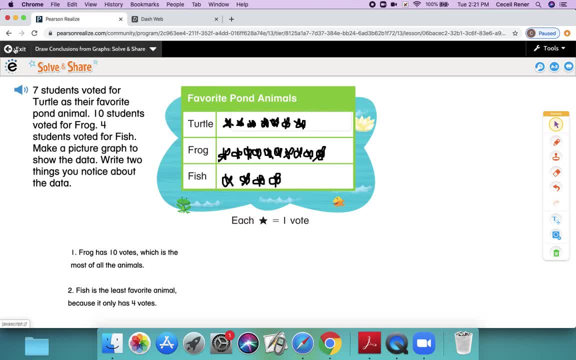 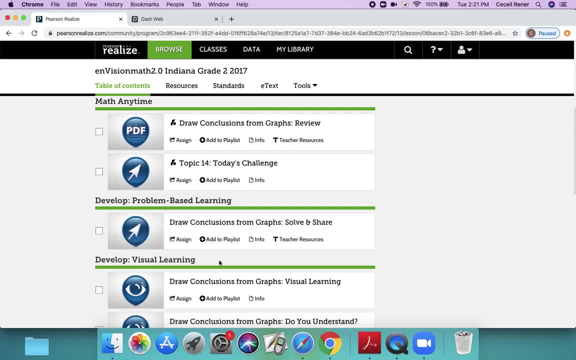 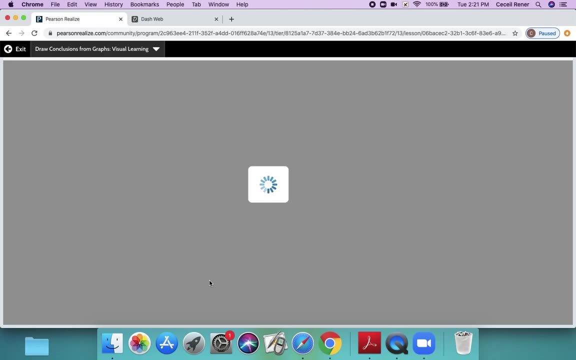 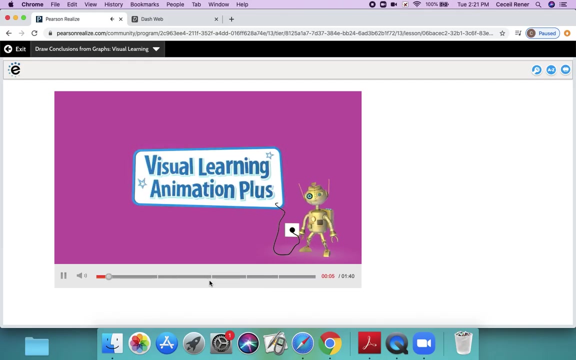 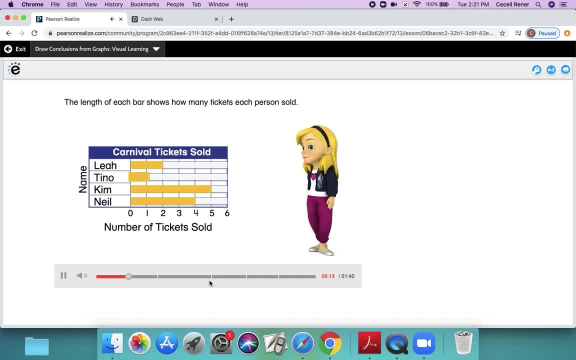 It's a bar graph. It's a bar graph. It's a bar graph. The length of each bar shows how many tickets each person sold. The student sold tickets to the carnival. How do you read the bars in the graph? Okay? 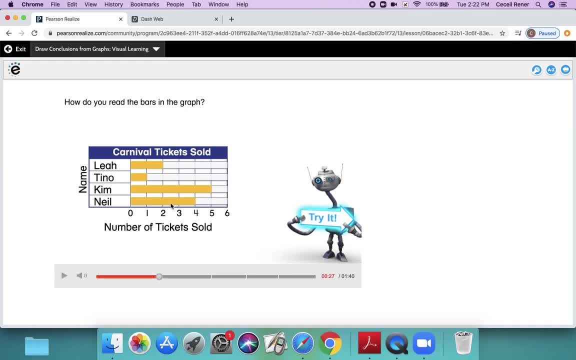 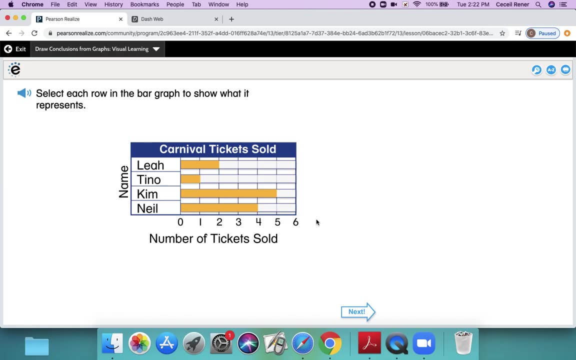 So how do we read the bars in the graph? What do we do here? Well, what do we do, boys and girls? I think we might as well just go to try it, because that's going to tell us We're going to go to where. 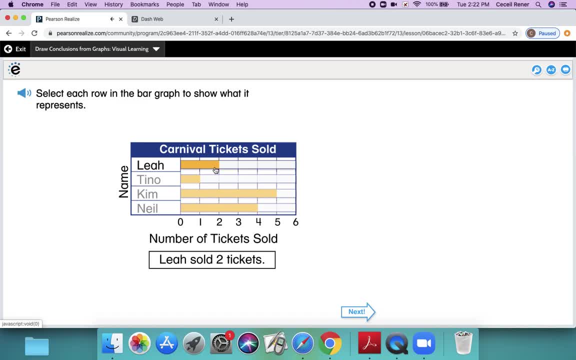 The end of the bar. Leah sold two tickets. Right, We go to the end of the bar and we look down. We followed the line all the way down. So Leah sold two tickets. Tino sold one ticket. We look at the end of the bar and we follow it down to the number of tickets sold and then we create one in the bottom. 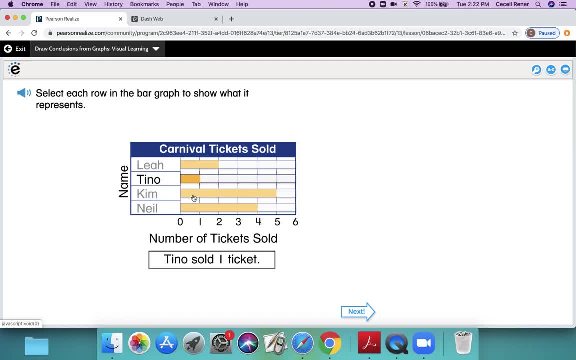 So we can draw a line in the back of each box. Where are the tickets? now we're to Kim, can you? I bet you already know how many tickets Kim sold? Kim sold five tickets. Neil sold four tickets. so we go to the end of the bar. 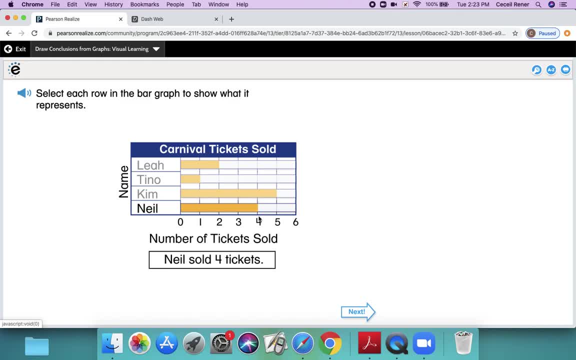 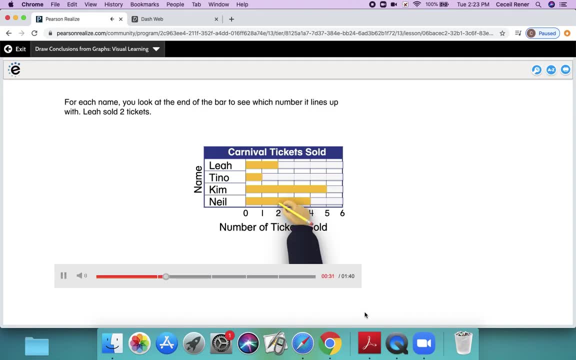 and we follow it down to the number sold for each name. you look at the end of the bar to see which number it lines up with. Leah sold two tickets. Tino sold one ticket. Kim sold five tickets. Neil sold four tickets. you can also compare information. who sold the most tickets. 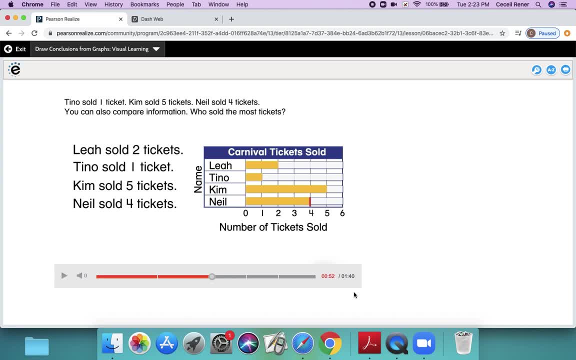 okay, so who sold the most tickets? so what we're going to do is we're going to look to see who has the longest bar. who is the longest bar? can you tell who has the longest bar so you compare the lengths of the bars? I think we can all see who has the longest bar. Kim sold the most tickets. who? 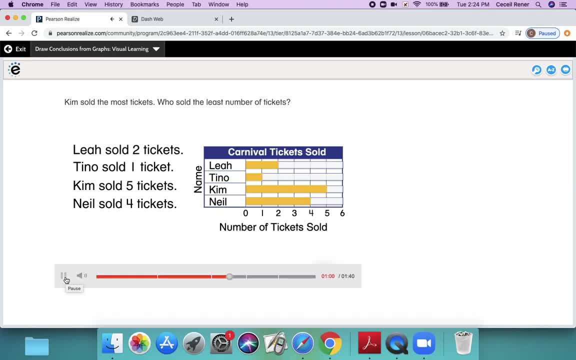 sold the least number of tickets. well, the least number of tickets, you know, sold the least number of tickets. how many more tickets did Kim sell than Tino? so you can figure this out by looking between Kim and Tino and seeing the difference between the bars. so we can count. we can count one, two, three, four. 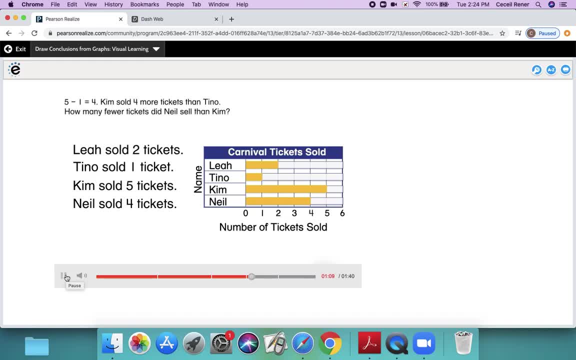 five minus one equals four. Kim sold four more tickets than Tino. how many fewer tickets did Neil sell, then Kim? Okay, so you can count the number of spaces, which would be one, or you could subtract it. Five minus four is one. It's the same either way. boys and girls. 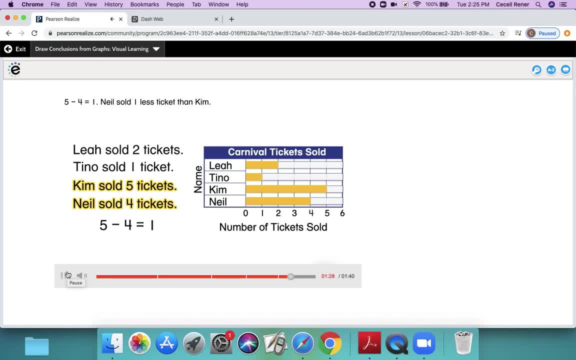 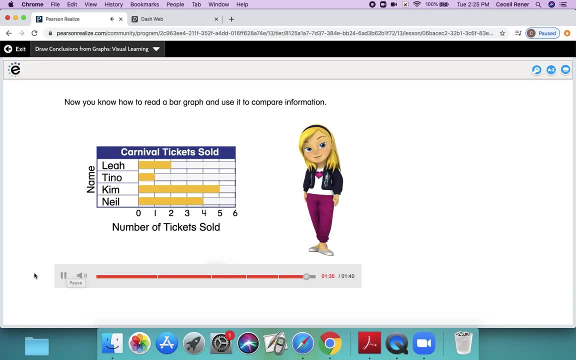 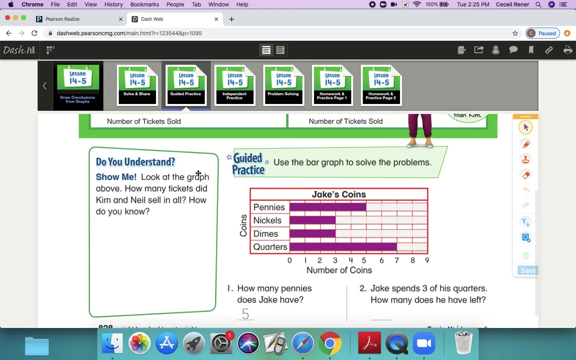 Five minus four equals one. Neil sold one less ticket than Kim. Now you know how to read a bar graph and use it to compare information. Okay, so now let's go to our book and let's talk about how we're going to use our bar. 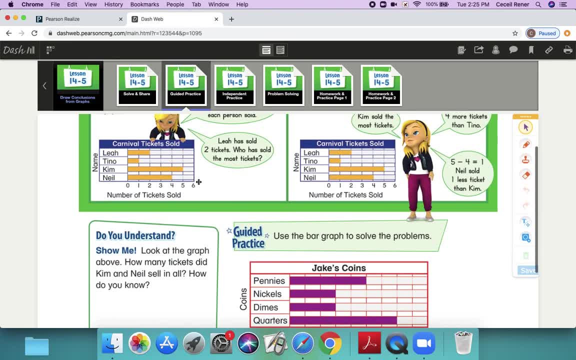 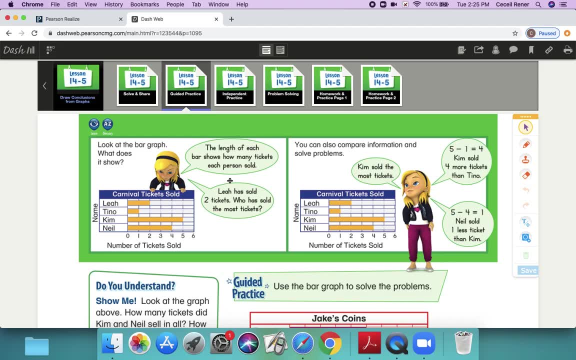 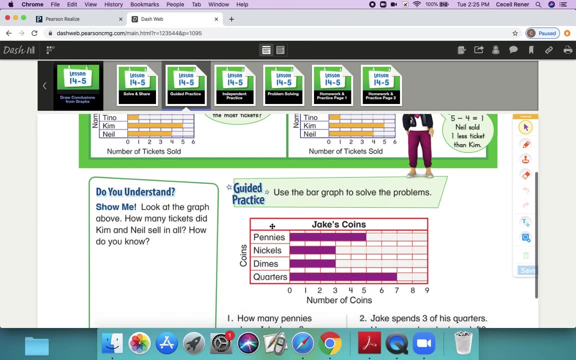 graph to solve the problems. As always, we can refer to the top of our page if we're confused and we're not sure what to do. It gives us the examples that were in our video. We can also go online. Let's go to our book and we're going to use the bar graph to solve the problems. 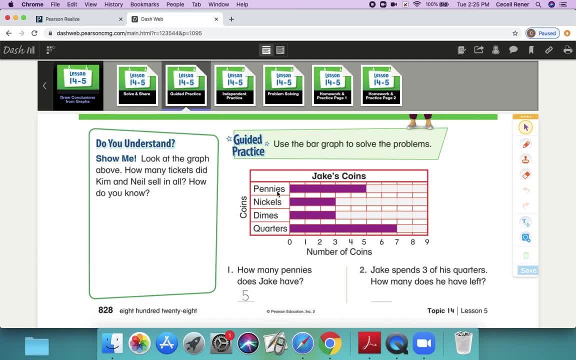 We have Jake's coins. The coins he has are listed here and it's labeled coins and then the number of coins are on the bottom. His coins range from zero to nine and he's got pennies, nickels, dimes and quarters. 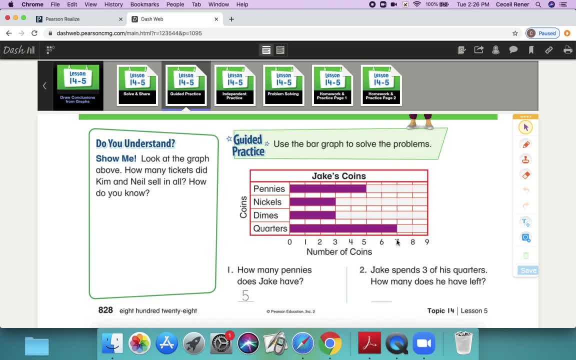 We can kind of visually look at it. We can see what he has the most of, what he's kind of: Oh, look at that, Look at the interesting thing about nickels and dimes, and then what's going on here. 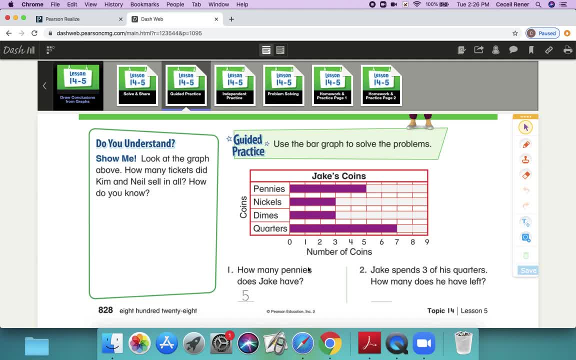 It says how many pennies does Jake have. We would go to the pennies, You would go where the bar ends and you would follow it down and we can see he has how many boys and girls. He has five. so I want you to trace over the five on your page. 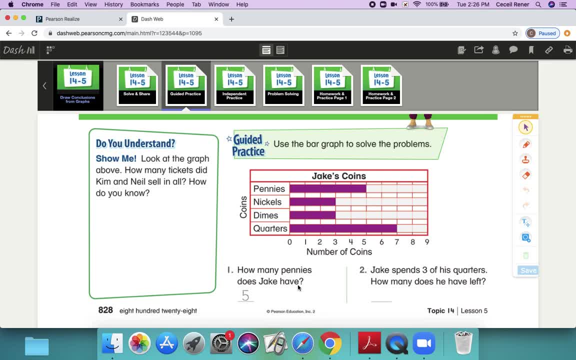 Trace that over. Now let's read questions. Question number two: Jake spends three of his quarters. How many does he have left? Let's go over here to the quarters Now he has. Let's see how many he has right now. 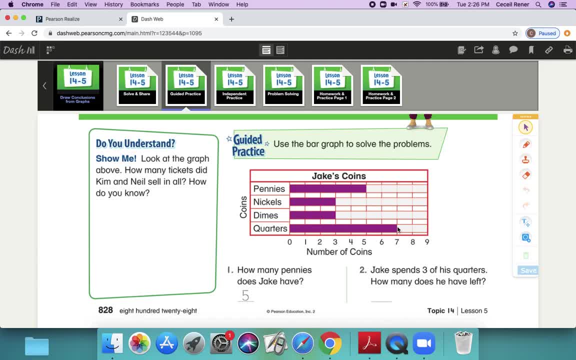 He has seven Now he spends three of them, so we're going to take away three. one, two, three. That leaves him with how many? Where does that leave us Right here? How many is that? That is four, so let's write four. 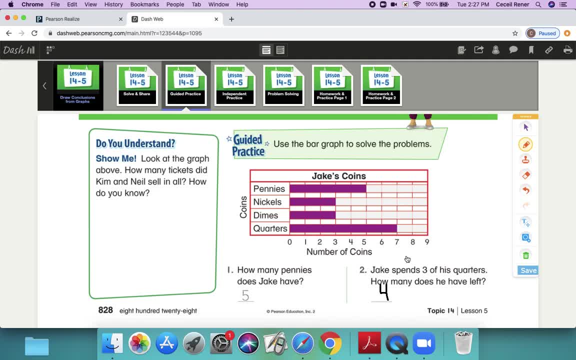 Because he had seven. seven minus three equals four. Seven minus three, oops, equals four. That's pretty basic. Okay, Let's go over here to the quarters. Okay, That's pretty basic. Now look at the graph above. 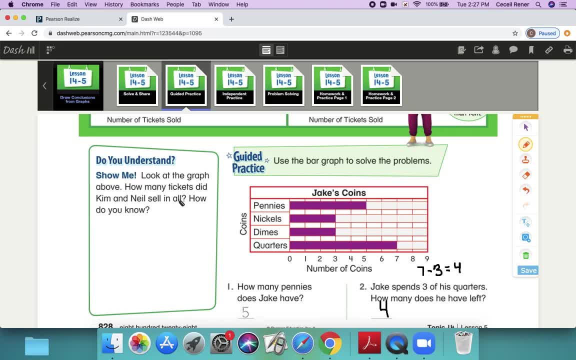 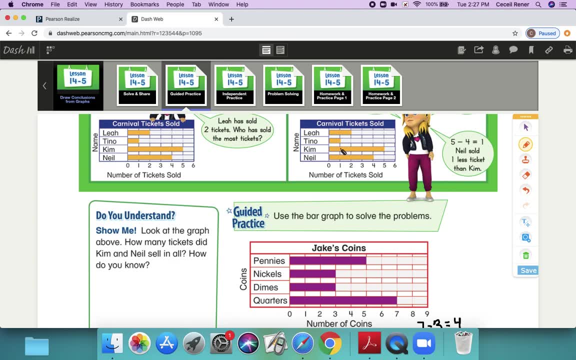 How many tickets did Kim and Neal sell in all? How do you know? So let's look at Kim and Neal. So we're going to go over here. Kim sold how many She sold. We look here. She sold five. Neal sold how many. 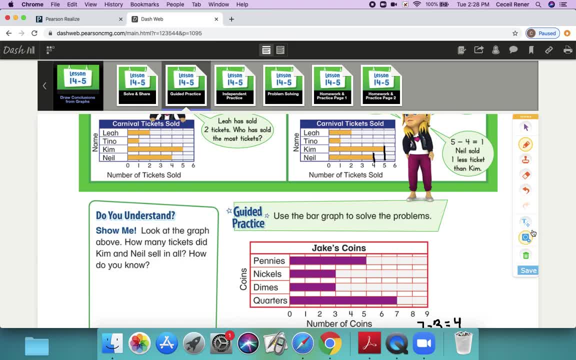 Four. So how many did they sell? Four? They sold nine. So we could say nine. And how do we know that? We know that Kim's bar goes to where Kim's bar goes to five. Kim's bar goes to five. 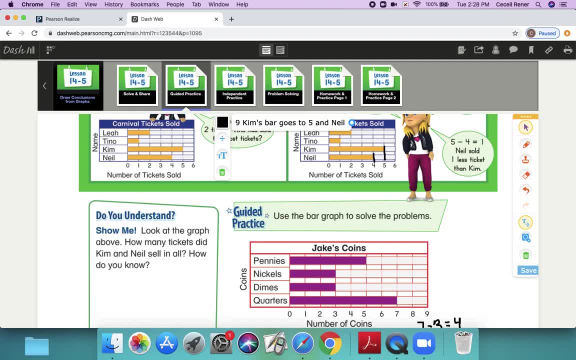 And Neal's bar Five. He's bar goes to four, Kim goes to five, Kim goes to three And Neal goes to three. He's bar runs to three. Kim goes to three. Again, it's all in order. It's 8 to 9 as well. 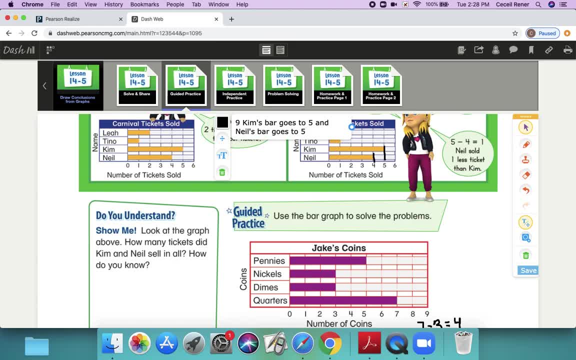 So 9,, 7,, 3, 4.. All right, So you've got the numbers here. You want to make a cross between the remove numbers? You want to do it again Now notice what we just did. You sometimes feel like you can make some crazy tens.